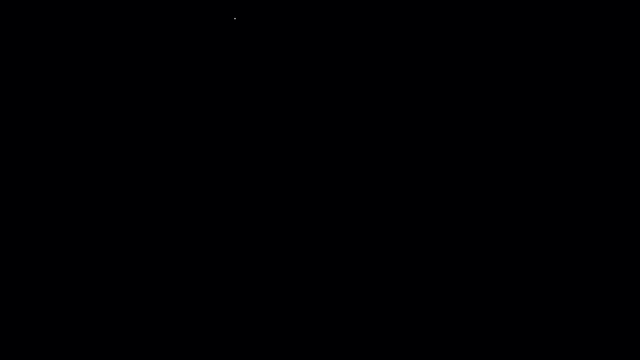 Let's try this problem. What is the limit, as x approaches 0, of the function? 5x divided by x squared plus 2x? Now we can't use direct substitution here, because if we plug in 0, we're going to have 0 divided by 0, which is indeterminate, so we're not going to do that. 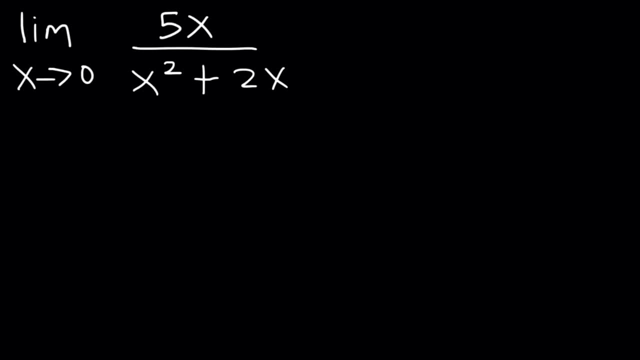 Instead we can evaluate this limit analytically by factoring. There's nothing to factor on the top, that is, on the numerator of the fraction, so we're not going to change it. But in the denominator we can take out the GCF, the greatest common factor. 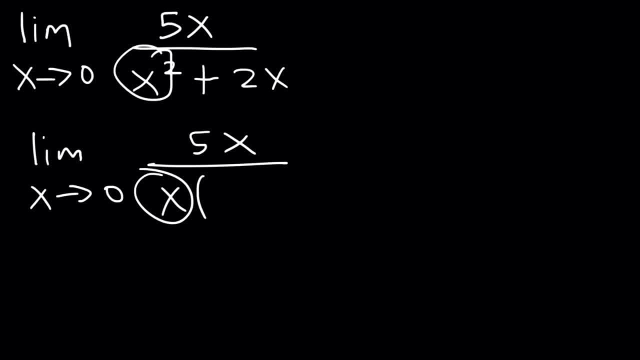 So if we take out an x, x squared divided by x is x, and 2x divided by x is positive 2.. Now notice that we can cancel an x variable, and so we'll be left with the limit, as x approaches 0 of 5 divided by x plus 2.. 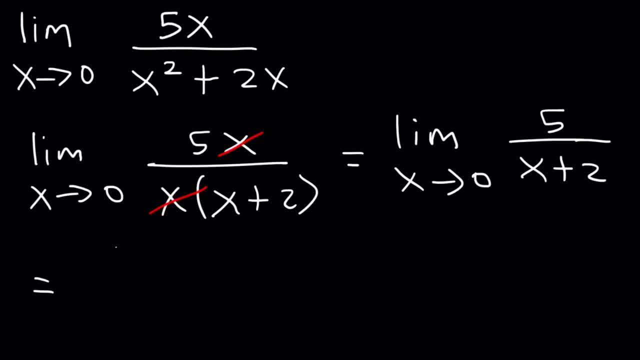 Now we can use direct substitution. Once you replace x with 0, there's no need to rewrite this limit expression. Now some teachers are picky about this, so you have to rewrite it until you replace x with this number. So the final answer is 0. 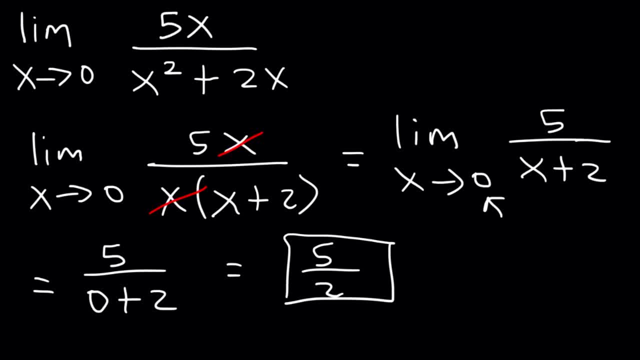 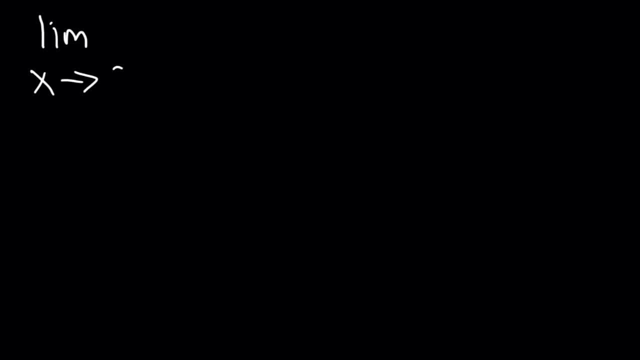 The final answer is 5 divided by 2.. That's the limit of this expression. Now what about this one? What is the limit, as x approaches 2, of x squared plus 3x minus 10 divided by x minus 2?? 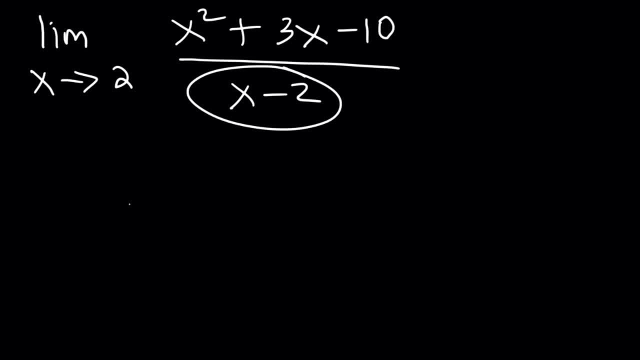 So we can't plug in a 2. If we do, we're going to get a 0 in the denominator and it's going to be undefined. So we've got to factor. How can we factor this trinomial? To do so, find two numbers that multiply to 10 but add to 3.. 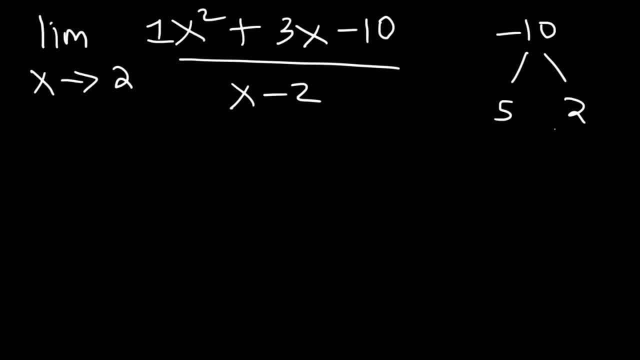 Two numbers that multiply to 10 are 5 and 2.. Now we can make it negative 5 and positive 2, or positive 5 and negative 2.. Now we want to make it positive 5 and negative 2, because those two numbers add up to positive 3.. 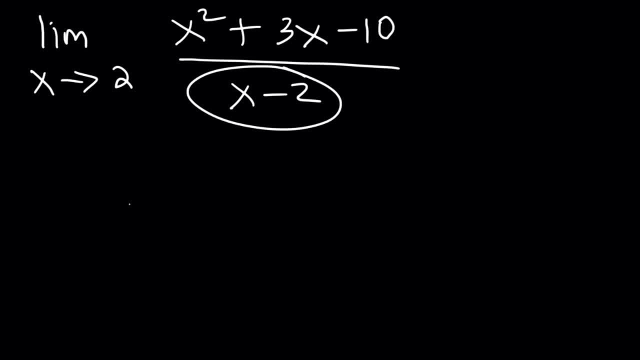 So we can't plug in a 2. If we do, we're going to get a 0 in the denominator and it's going to be undefined. So we've got to factor. How can we factor this trinomial? To do so, find two numbers that multiply to 10 but add to 3.. 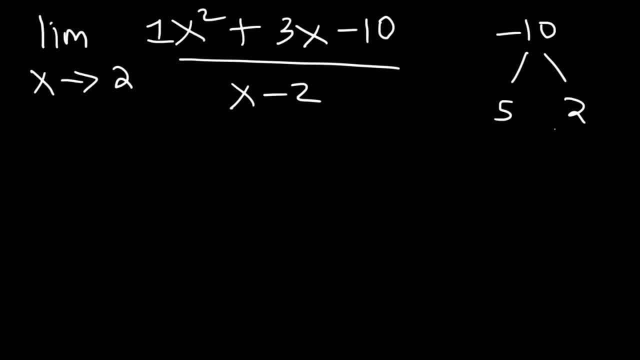 Two numbers that multiply to 10 are 5 and 2.. Now we can make it negative 5 and positive 2, or positive 5 and negative 2.. Now we want to make it positive 5 and negative 2, because those two numbers add up to positive 3.. 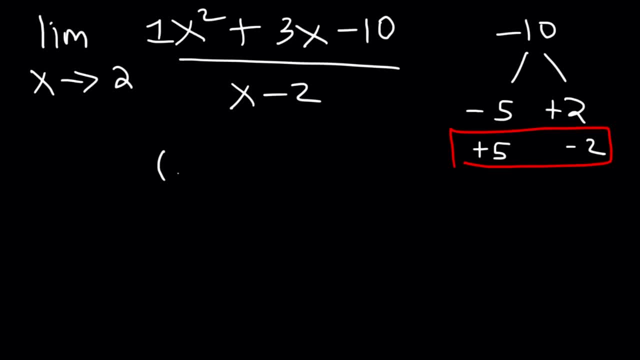 So therefore, x squared plus 3x minus 10 can be factored As x plus 5 times x minus 2.. And we need to rewrite the limit expression So notice that we can cancel the factor x minus 2.. And so we're left with the limit, as x approaches 2, of x plus 5.. 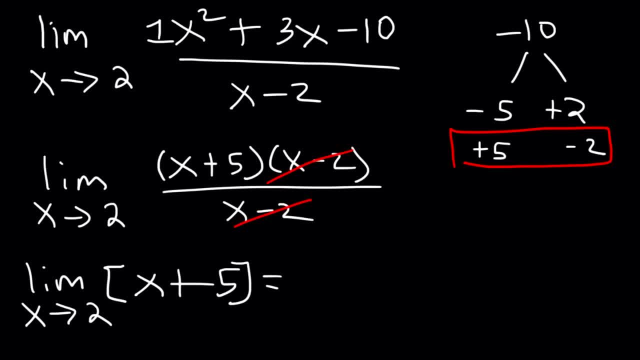 So now we can use direct substitution. We're not going to get a 0 in the denominator anymore, So it's going to be 2 plus 5, which is 7.. So that's the limit. Here's another problem that you could try. 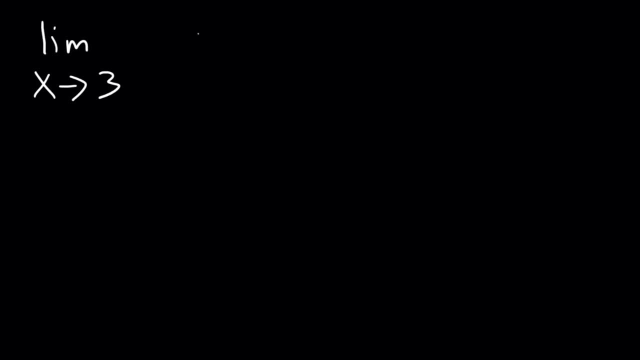 What is the limit, as x approaches 3, of x squared minus 9, divided by x minus 3?? So what do you think What is the answer to this problem? Well, we need to factor x squared minus 9 and we can use the difference of perfect squares. 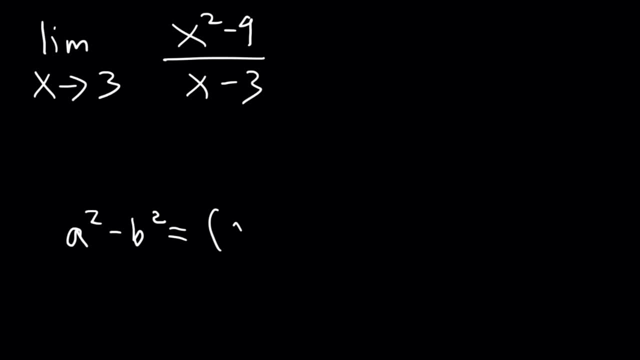 formula. So, for example, if you have a squared minus b squared, it's going to be a plus b times a minus b. So, for example, let's say if we have x squared minus 25.. The square root of x squared is x, the square root of 25 is 5, and one is going to be positive. 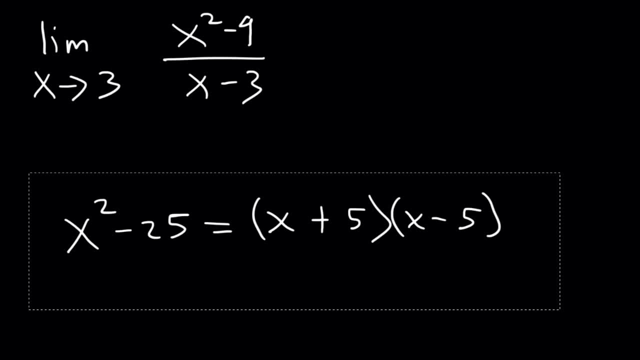 and the other is going to be negative. That's how you can factor it. So, for the example that we have, Okay, The square root of x, squared as we said before, is x and the square root of 9 is 3.. 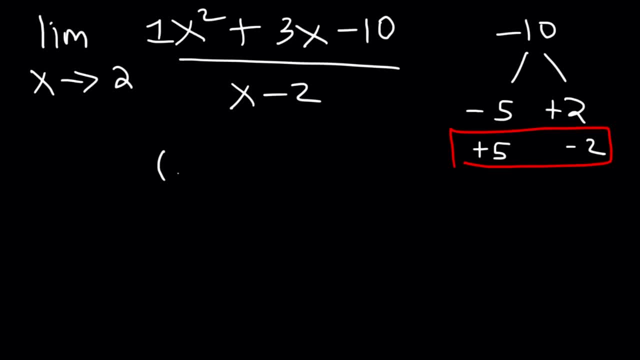 So therefore, x squared plus 3x minus 10 can be factored. Now we need to rewrite the limit expression So notice that we can cancel the factor x minus 2.. And so we're left with the limit, as x approaches 2, of x plus 5.. 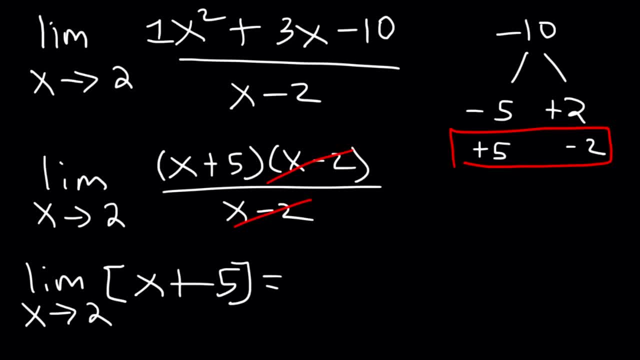 So now we can use direct substitution. We're not going to get a 0 in the denominator anymore, So it's going to be 2 plus 5, which is 7.. So that's the limit. Here's another problem that you could try. 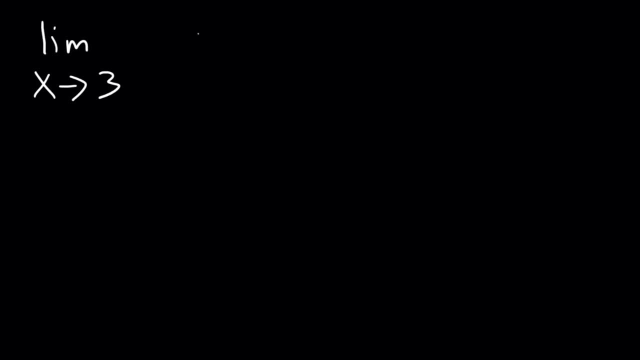 What is the limit, as x approaches 3, of x squared minus 9, divided by x minus 3?? So what do you think What is the answer to this problem? Well, we need to factor x squared minus 9 and we can use the difference of perfect squares. 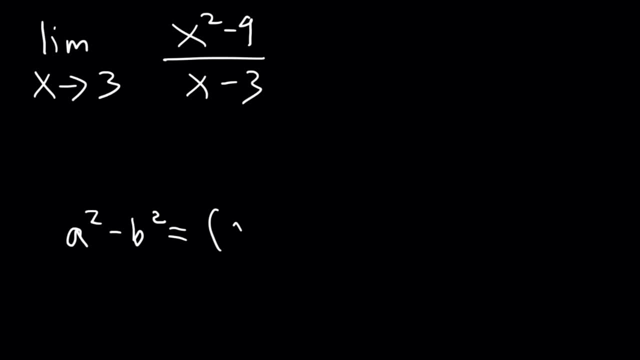 formula. So, for example, if you have a squared minus b squared, it's going to be a plus b times a minus b. So, for example, let's say if we have x squared minus 25.. The square root of x squared is x, the square root of 25 is 5, and one is going to be positive. 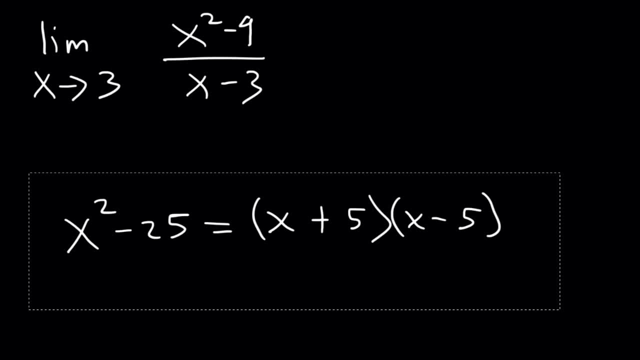 and the other is going to be negative. That's how you can factor it. So, for the example that we have, Okay, The square root of x, squared as we said before, is x and the square root of 9 is 3.. 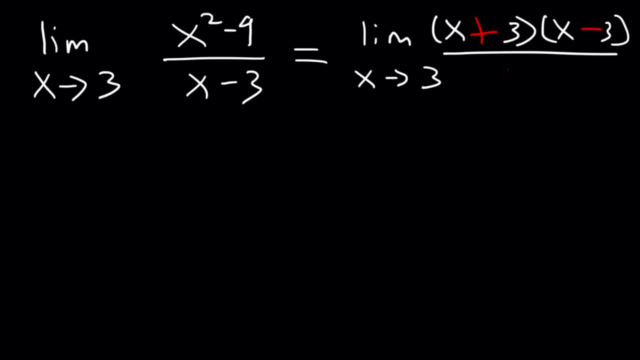 And so it's going to be x plus 3 and x minus 3.. So we can cancel with the 3 on the bottom, And now we're left over with the limit, as x approaches 3, of x plus 3.. And now let's use direct substitution. 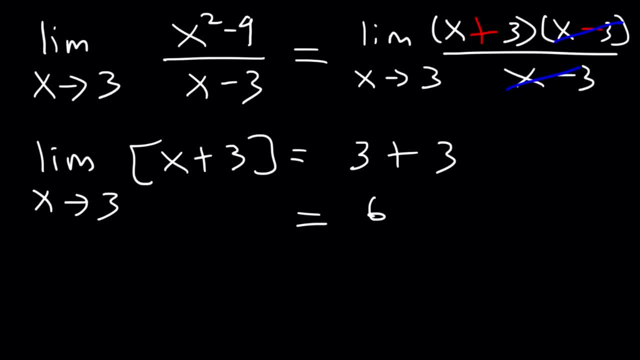 So it's going to be 3.. So it's going to be 3 plus 3,, which is equal to 6.. And so that's how we can evaluate this particular limit. What is the limit, as x approaches 2, of x cubed minus 8 divided by x minus 2?? 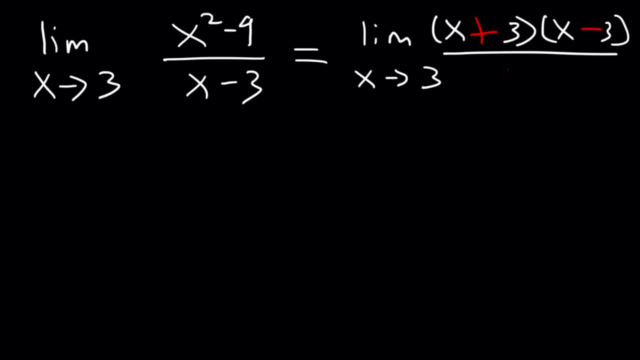 And so it's going to be x plus 3 and x minus 3.. So we can cancel with the 3 on the bottom, And now we're left over with the limit, as x approaches 3, of x plus 3.. And now let's use direct substitution. 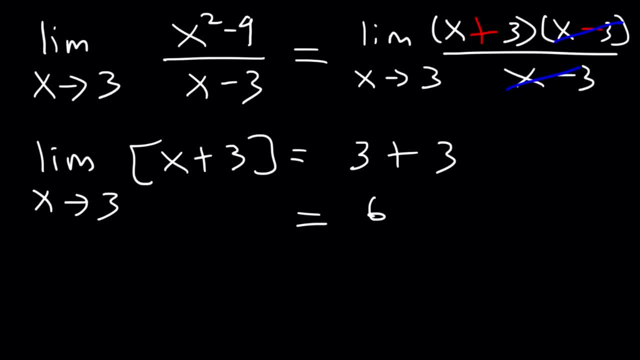 So it's going to be 3.. It's going to be 3 plus 3,, which is equal to 6.. And so that's how we can evaluate this particular limit. What is the limit, as x approaches 2, of x cubed minus 8 divided by x minus 2?? 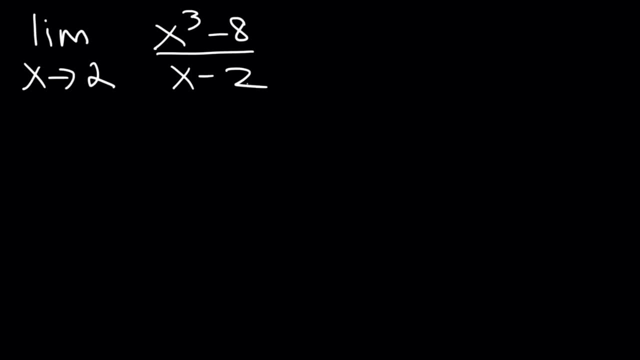 What would you do in that case? So what we need to do is factor this, We need to do the difference of perfect cubes, And the formula that we need to use is this: one a cubed minus b cubed is a minus b times. 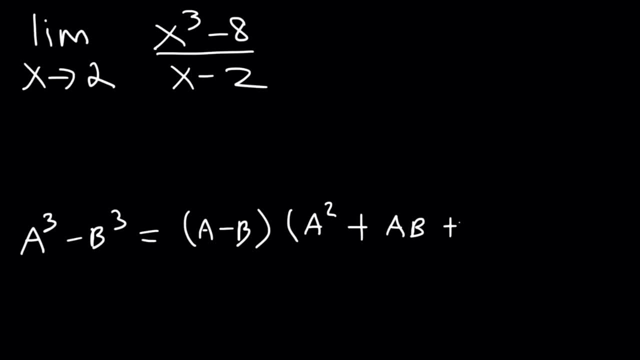 a squared plus ab plus b squared. So in this case a cubed is x cubed, B to the third is 8.. So a is the cube root of x cubed, which is x, and b is the cube root of 8, which is 2.. 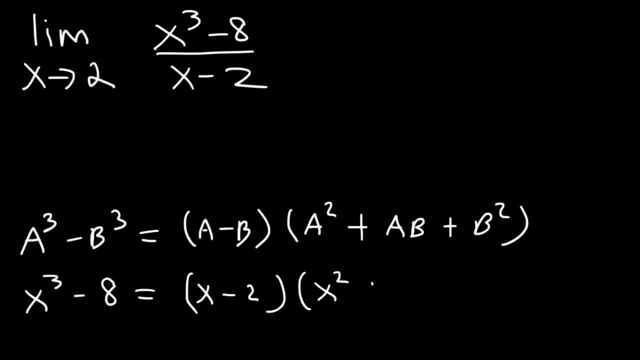 a squared, That's x times 2.. That's x times x, which is x squared. ab, that's x times 2, or 2x And b squared is 2 squared, which is 4.. So therefore, we have the expression, the limit as x approaches 2, x minus 2 times x squared. 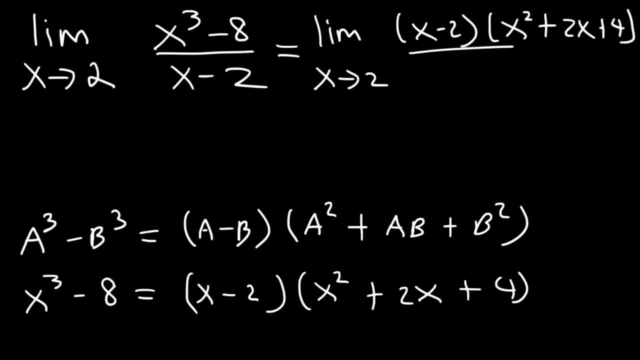 plus 2x plus 4 divided by x minus 2.. All right, Let's get rid of this stuff on the bottom, And now we can cancel the x minus 2 factor. So we have the limit, as x approaches 2, of this remaining expression. 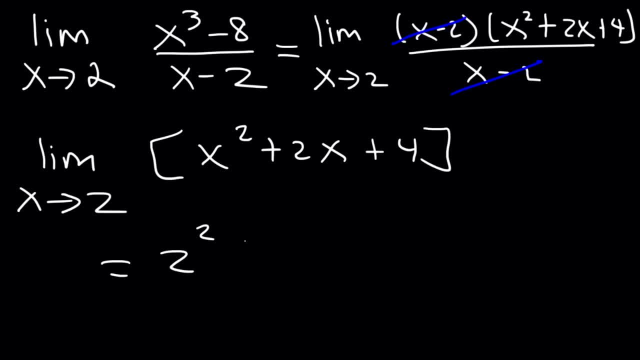 And now let's use a direct substitution. So this is equal to 2 squared plus 2 times 2 plus 4.. 2 squared is 4, 2 times 2 is 4.. And 4 plus 4 plus 4 three times is the same as 4 times 3, which is 12.. 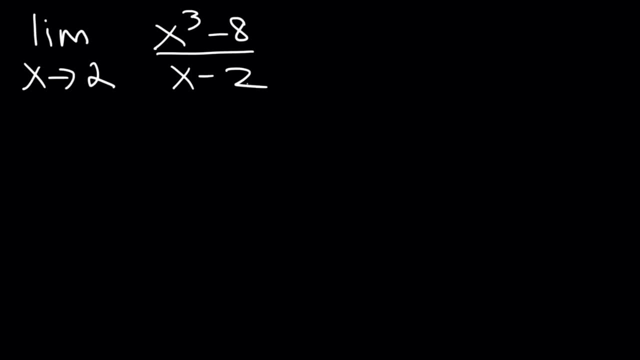 What would you do in that case? So what we need to do is factor, We need to do the difference of perfect cubes, And the formula that we need to use is this: one a cubed minus b cubed is a minus b times. 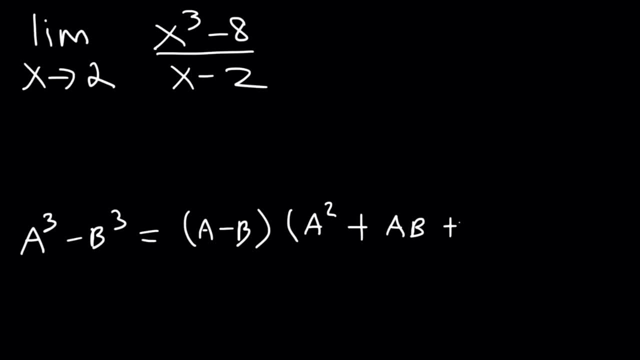 a squared plus ab plus b squared. So in this case a cubed is x cubed, B to the third is 8.. So a is the cube root of x cubed, which is x, and b is the cube root of 8, which is 2.. 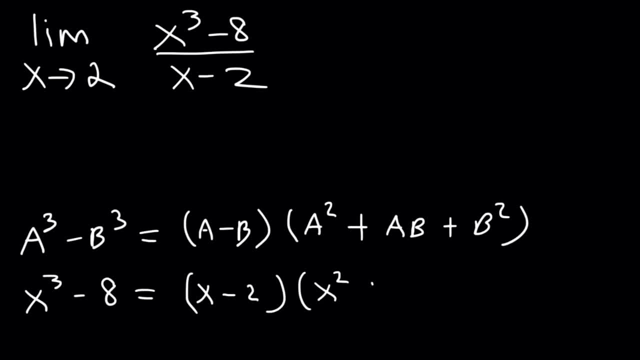 a squared, That's x times 2.. That's x times x, which is x squared. ab, that's x times 2, or 2x And b squared is 2 squared, which is 4.. So therefore, we have the expression, the limit as x approaches 2, x minus 2 times x. 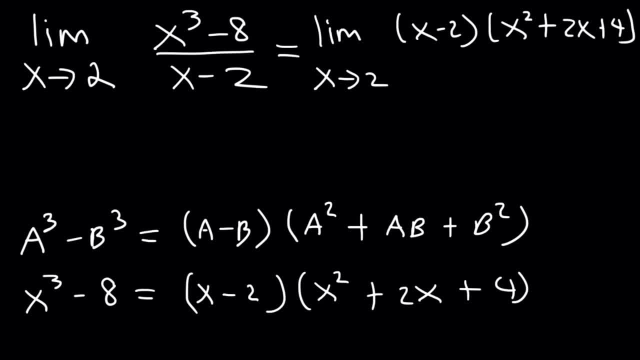 squared plus 2x plus 4, divided by x minus 2.. All right, Let's get rid of this stuff on the bottom, And now we can cancel the x minus 2 factor. So we have the limit as x approaches 2 of this remaining expression. 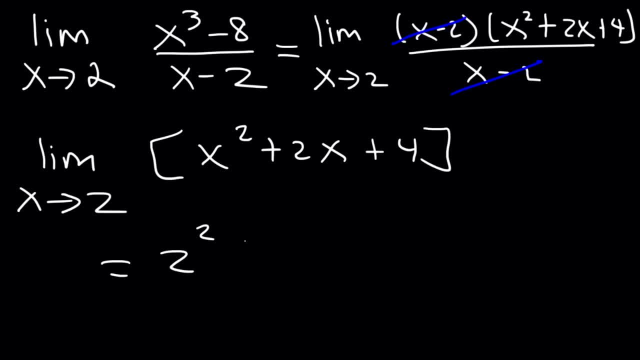 And now let's use a direct substitution. So this is equal to 2 squared plus 2 times 2 plus 4.. 2 squared is 4, 2 times 2 is 4.. And 4 plus 4 plus 4 three times is the same as 4 times 3, which is 12.. 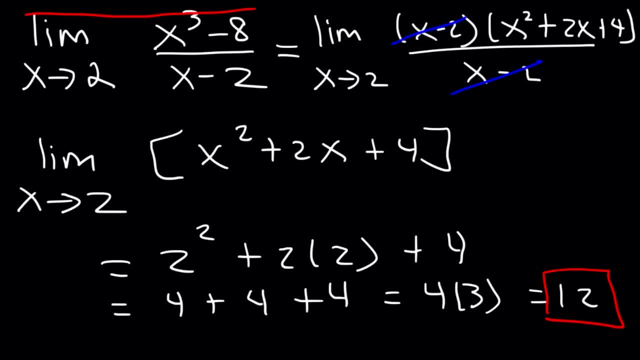 And so that's the limit as x approaches 2.. All right, We now know how to obtain the element of this expression, So we need to be familiar with the different factoring techniques that you've learned in a typical algebra course. Now let's try this one. 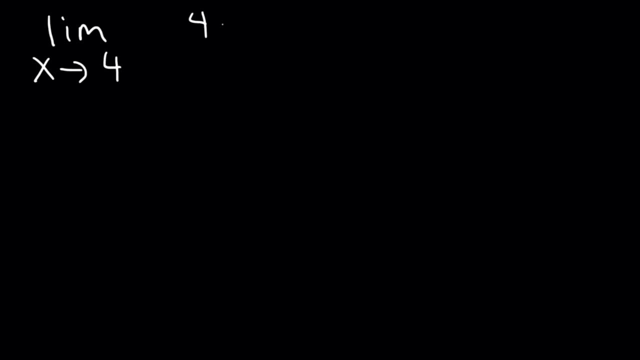 What is the limit? as x approaches 4 of 4 minus x divided by x squared minus 16.. So take a minute and pause the video, See if you can get this one right. So what do you think we need to do here? 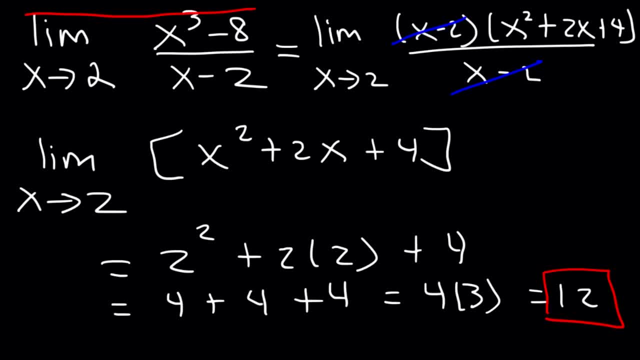 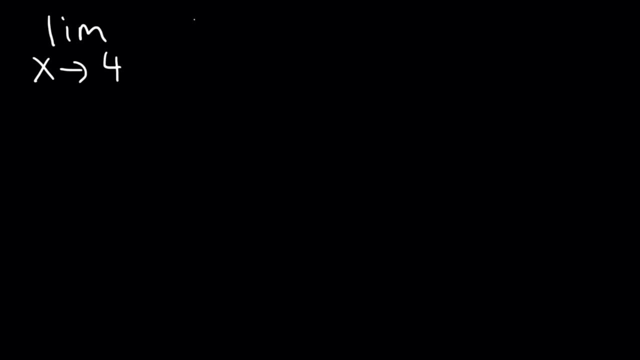 And so that's the limit as x approaches 2.. So this expression. So you need to be familiar with the different factoring techniques that you've learned in a typical algebra course. Now let's try this one. What is the limit as x approaches 4 of 4 minus x divided by x squared minus 16?? 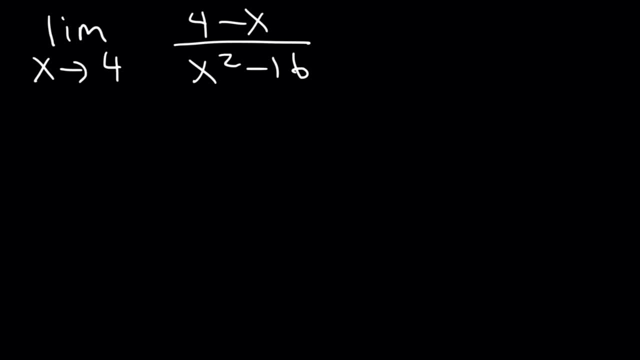 So take a minute and pause the video, See if you can get this one right. So what do you think we need to do here? So looking at x squared minus 16.. We can see we have a difference of perfect squares situation. So to factor it, it's going to be x plus 4 times x. 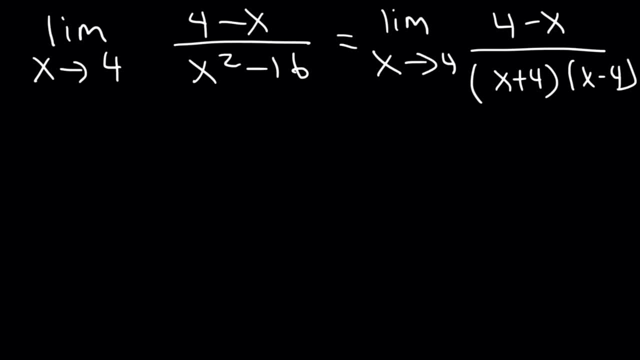 minus 4.. But 4 minus x and x minus 4, they don't really cancel at the present moment. However, what we can do is factor out a negative 1.. If we take out a negative 1 in the front and then 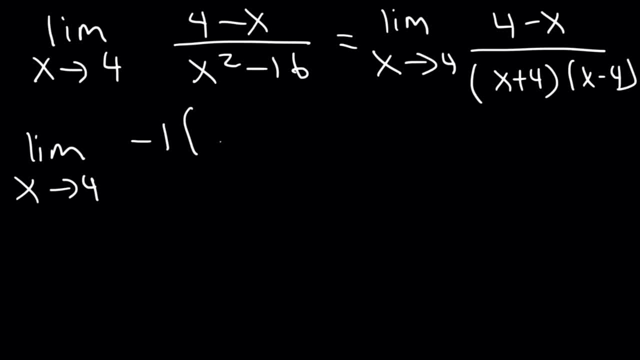 reverse the order of 4 minus x. notice that if you take a negative from negative x, you're going to get positive x. If you take a negative from positive 4, it changes to negative 4.. So by factoring out a negative 1, we now can cancel x minus 4.. 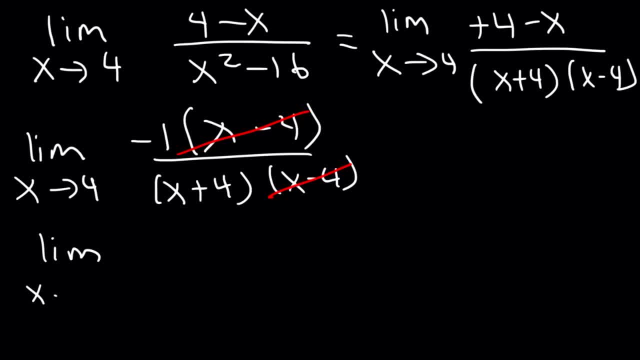 And so what we have left over is the limit, as x approaches 4, of negative 1 divided by x plus 4.. And so this is going to be negative 1 over x minus 4.. Over 4 plus 4, and 4 plus 4 is 8.. So the answer is negative 1 divided by 8.. 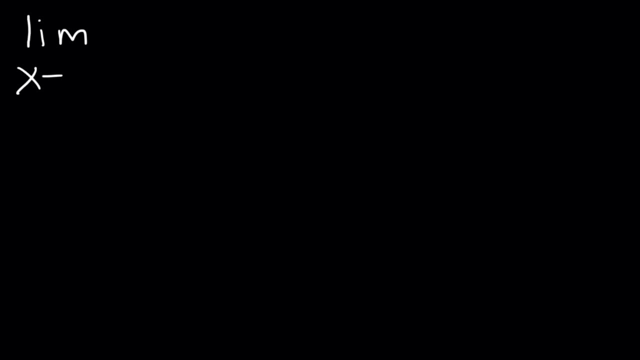 Now what is the limit, as x approaches 4, of the expression x squared minus x minus 12, divided by x squared plus x minus 20?? So we just need to factor completely. Let's go ahead and do that. Let's go ahead and factor this expression. So what two numbers multiply to negative 12? 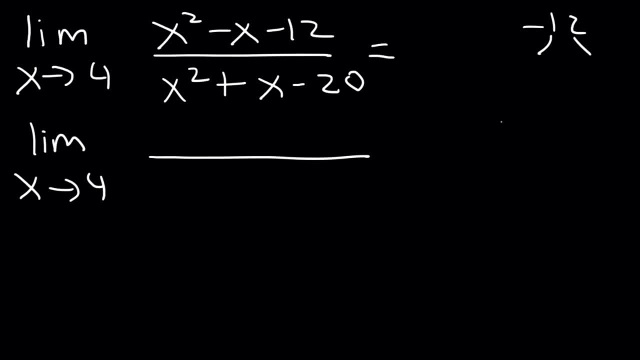 but add to the middle coefficient negative 1?. So we know 4 times 3 is 12, but we need to make the 4 negative, because negative 4 plus positive 3 is negative 1.. So this is going to be x minus 4. 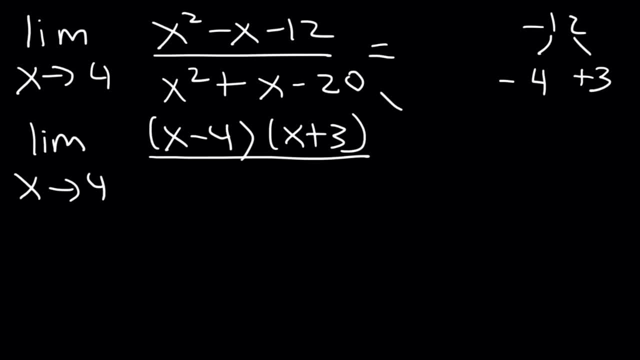 times x plus 3.. Now what two numbers multiply to negative 20 but add to 1? Well, we know, 5 times 4 is 20, but we need to make it positive 3.. So we need to make the 4 negative, 4 plus positive 3 is. 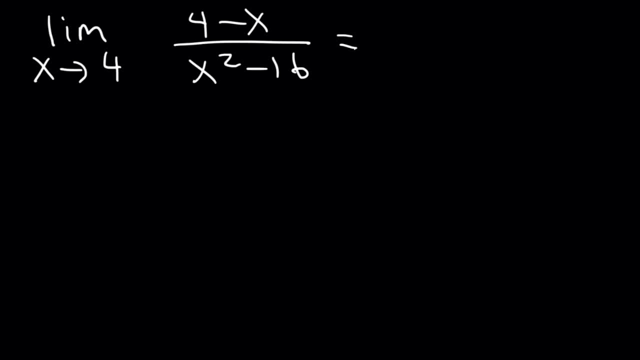 So, looking at x squared minus 16. 12. we have a difference of perfect squares situation. So to factor it, it's going to be x plus 4 times x minus 4.. But 4 minus x and x minus 4, they don't really cancel at the present moment. However, what we can do is factor out a negative 1. If we take out a negative 1 in the front and then reverse the order of 4 minus x, notice that if you take a 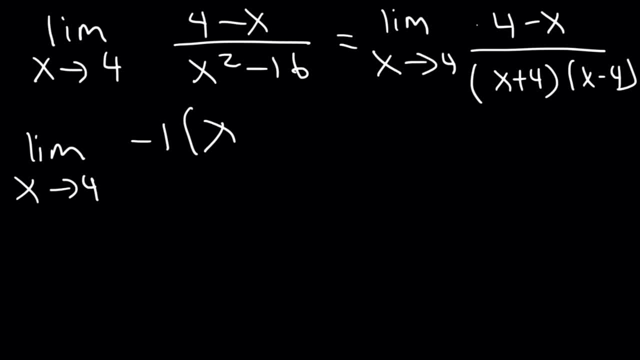 negative from negative x, you're going to get positive x. If you take a negative from positive 4, it changes to negative 4.. So by factoring out a negative 1, we now can cancel x minus 4.. And so what we have left over is the limit, as x approaches 4, of negative 1 divided by x plus 4.. And so this is going to be negative 1 over 4 plus 4, and 4 plus 4 is 8.. 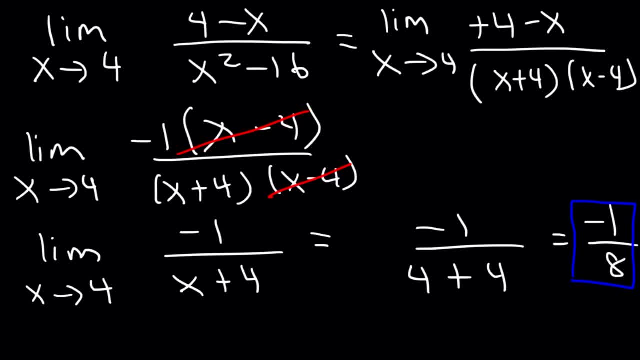 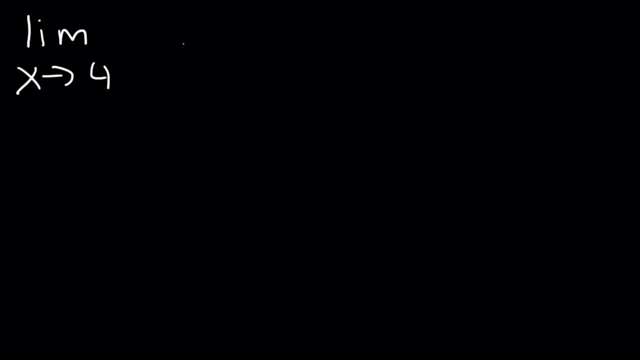 So the answer is negative: 1 divided by 8.. Now what is the limit, as x approaches 4, of the expression x squared minus x minus 12, divided by x squared plus x minus 20?? So we just need to factor completely. Let's go ahead and factor this expression. 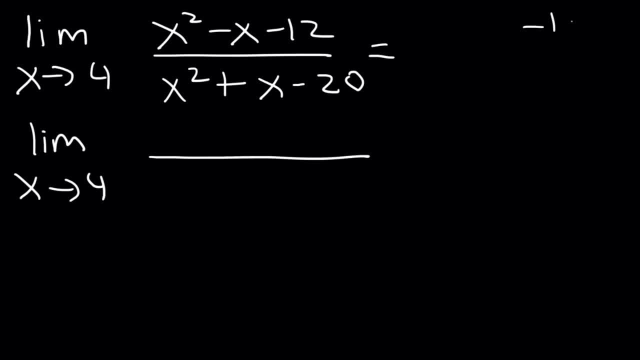 So what 2 minus x is? So what 2 numbers multiply to negative 12, but add to the middle coefficient negative 1? So we know 4 times 3 is 12, but we need to make the 4 negative, because negative 4 plus positive 3 is negative 1.. So this is going to be x minus 4 times x plus 3.. Now what 2 numbers multiply to negative 20, but add to 1? Well, we know 5 times 4 is 20, but we need to make it positive 5 and negative 4, because that's going to add up to 1.. 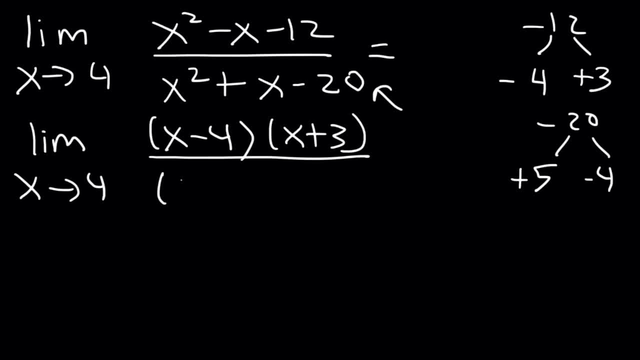 positive 5 and negative 4, because that's going to add up to 1.. So it's x plus 5 times x minus 4.. So we can cancel x minus 4.. And so we're left with the limit, as x approaches 4, of x plus 3. 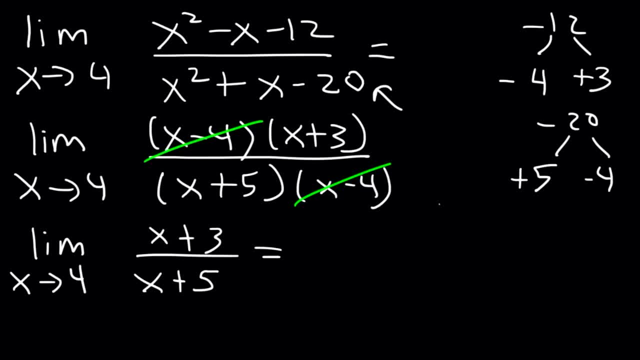 divided by x plus 5.. So if we plug in 4, it's going to be 4 plus 3 over 4 plus 5.. Now, 4 plus 3, we know it's 7.. 4 plus 5 is 9.. 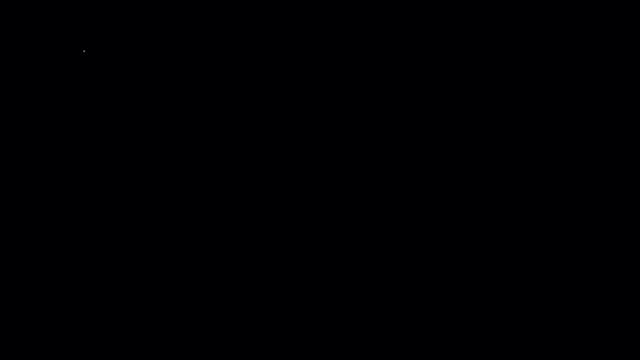 So that's the answer: 7 divided by 9.. What is the limit, as x approaches negative 1, of the expression 2x squared minus x minus 3 over x plus 1?? So what can we do here? What would you do? 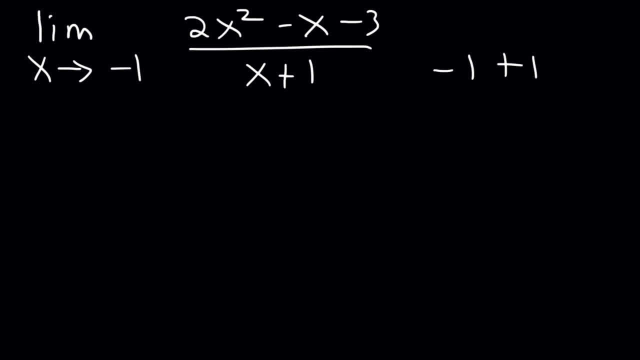 So first, we can't plug in negative 1, because on the bottom it's going to give us 0, and so that's undefined. But we need to factor this trinomial, But notice that the leading coefficient is not 1. So the way in which we factor it is going to be different. So first, 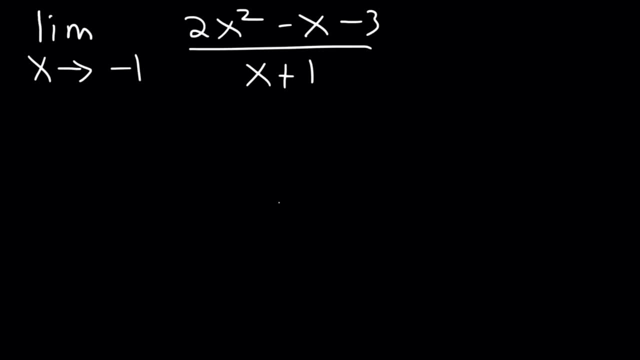 let's multiply 2 times negative 3.. 2 times negative 3 is negative 6. What two numbers multiply to negative 6, but add to the middle coefficient of negative 1? This is going to be negative 3 and 2.. So to factor it, we're going to replace the middle term. 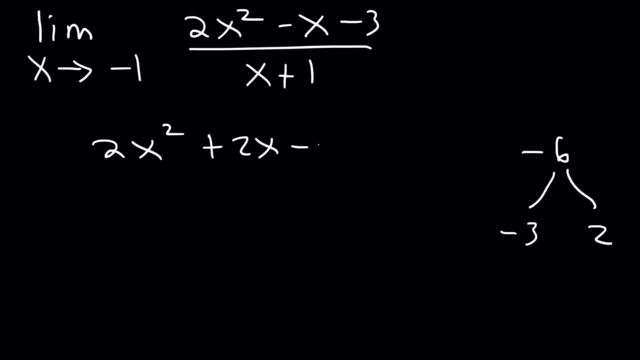 negative x with positive 2x minus 3x. Next, let's factor by grouping. In the first two terms, take out the GCF, which is 2x, And so you'd be left with x plus 1.. In the last two terms: 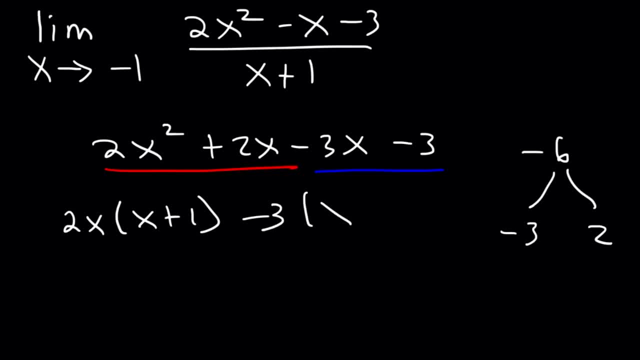 take out the greatest common factor, which is negative 3. And so you're going to get x plus 1.. Next, factor out x plus 1.. So we're going to write it once If we take out x plus 1 from the first. 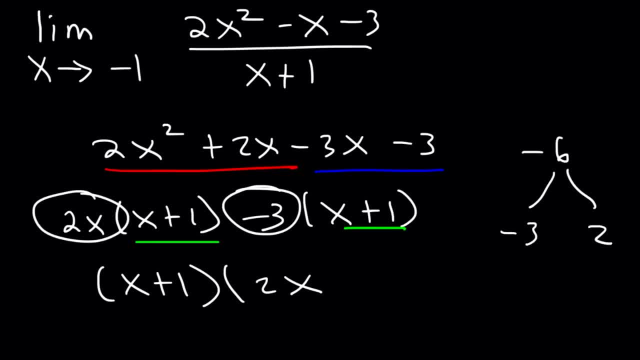 term, we'll be left with 2x, And so we're going to get x plus 1.. And so we're going to write it once. If we take it out from the second term, we're going to have negative 3 left over. 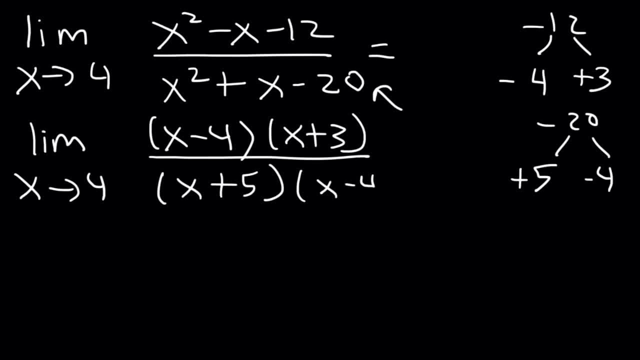 x plus 5 times x minus 4.. So we can cancel x minus 4.. And so we're left with the limit as x approaches: 4 of x plus 3 divided by x plus 5.. So if we plug in 4, it's going to be 4 plus 3 over 4 plus 5.. Now 4 plus 3, we know it's 7.. 4 plus 5 is 9.. And so that's the answer: 7 divided by 9.. 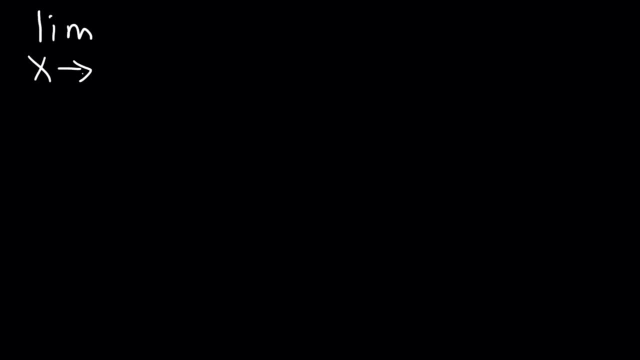 What is the limit, as x approaches negative 1, of the expression 2x squared minus x minus 3 over x plus 1?? So what can we do here? What would you do? So first, we can't plug in negative 1, because on the bottom it's going to give us 0. And so that's undefined. 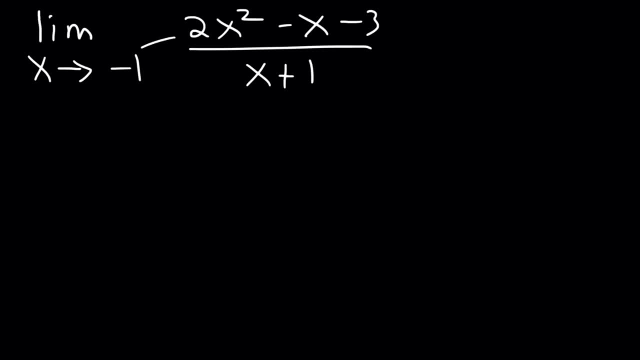 But we need to factor this trinomial But notice that the leading coefficient is not 1. So the way in which we factor it is going to be different. So first let's multiply 2 times negative 3.. 2 times negative 3 is negative 6. What 2 numbers multiply to negative 6 but add to the middle coefficient of negative 1?? 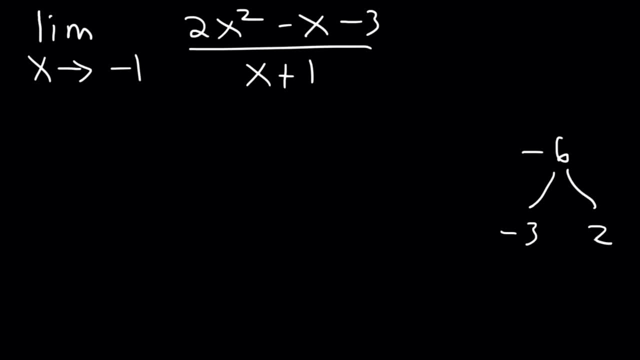 This is going to be negative 3 and 2.. So to factor it, we're going to replace the middle term negative x with positive 2x minus 2x. Next, let's factor by grouping In the first two terms. take out the GCF, which is 2x, And so you'd be left with x plus 1.. 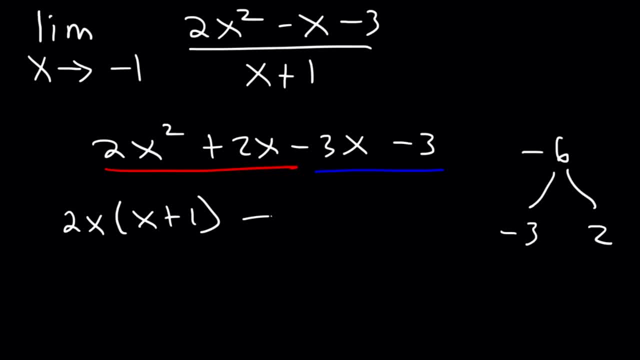 In the last two terms. take out the greatest common factor, which is negative 3.. And so you're going to get x plus 1.. Next factor out: x plus 1.. So we're going to write it once: If we take out x plus 1 from the first term, we'll be left with 2x. 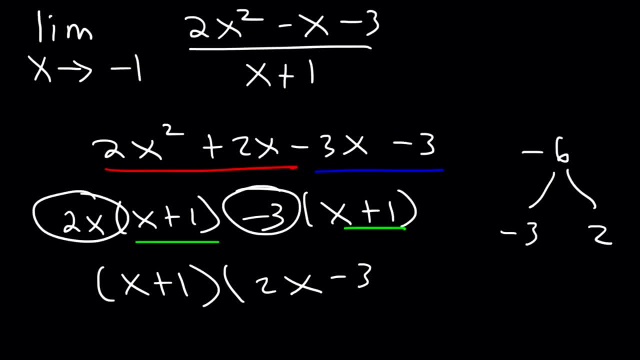 If we take it out from the second term, we're going to have negative 3x. So therefore we can say this is equal to the limit as x approaches negative 1, x plus 1, times 2x minus 3, divided by x plus 1.. 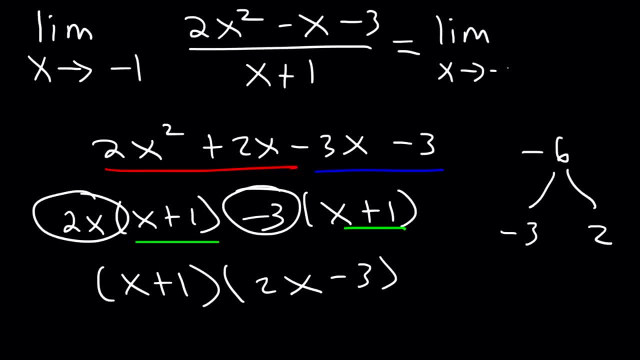 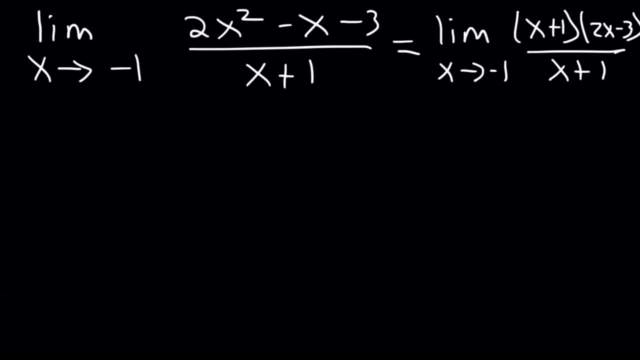 So therefore we could say: this is equal to the limit as x approaches negative 1, x plus 1 times 2x minus 3 divided by x plus 1.. So now we can cancel x plus 1.. And so we're left with the limit as x approaches negative 1.. 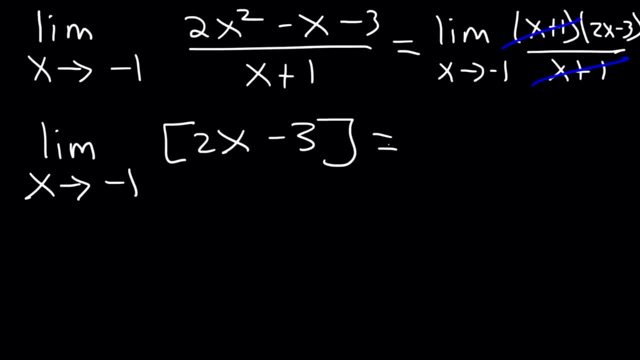 Of 2x minus 3.. So now let's use direct substitution. So this is going to be 2 times negative, 1 minus 3, which is negative 2 minus 3. And that's equal to negative 5.. So that's the final answer. 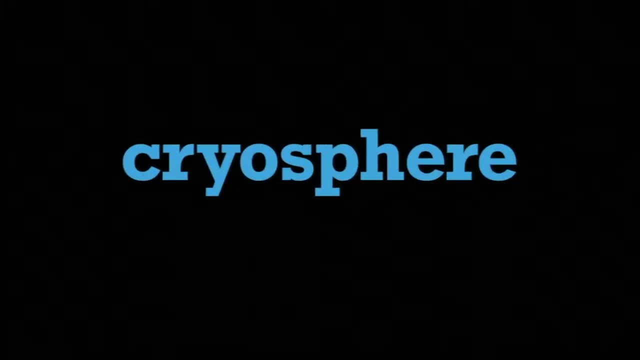 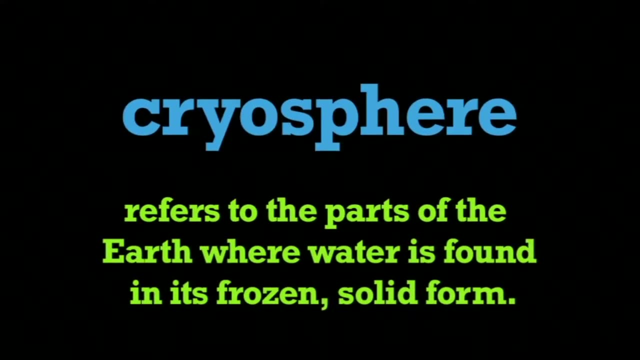 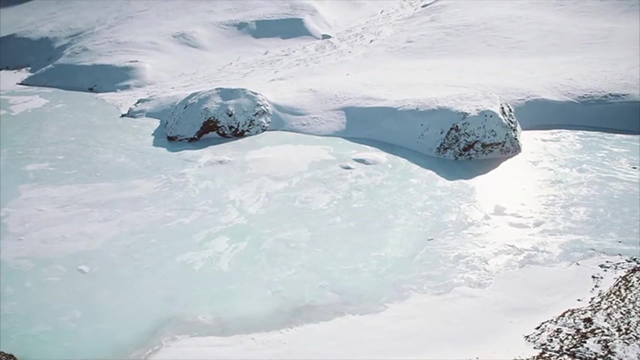 In this program we're going to discuss the cryosphere. What is the cryosphere? The term cryosphere refers to the parts of the earth where water is found in its frozen solid form. The cryosphere comprises frozen lakes, glaciers, sea ice. 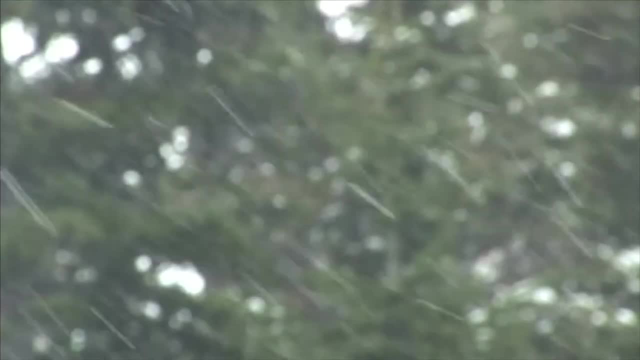 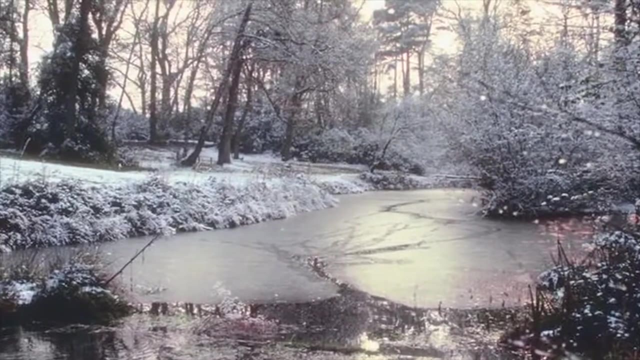 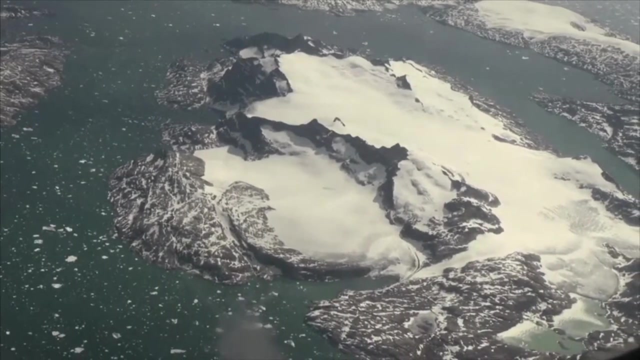 icebergs, snow, ice caps and permafrost soils. Snow and ice found on ponds and lakes are part of the cryosphere only during the winter months. Glaciers and ice caps are frozen year-round, and many can remain solid for tens of thousands. 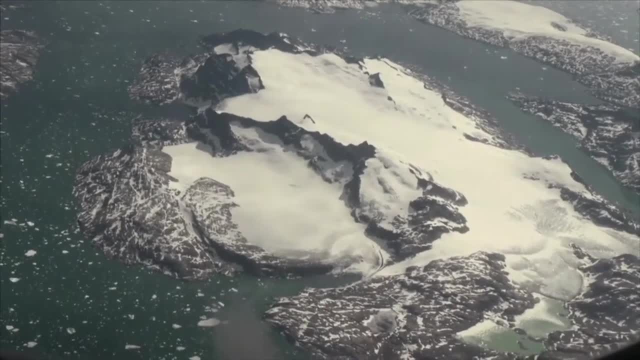 of years. The word cryosphere comes from the Greek cryos, which means cold, ice and snow. The word cryosphere comes from the Greek cryos, which means cold, ice and snow. The word cryosphere comes from the Greek cryos, which means cold. 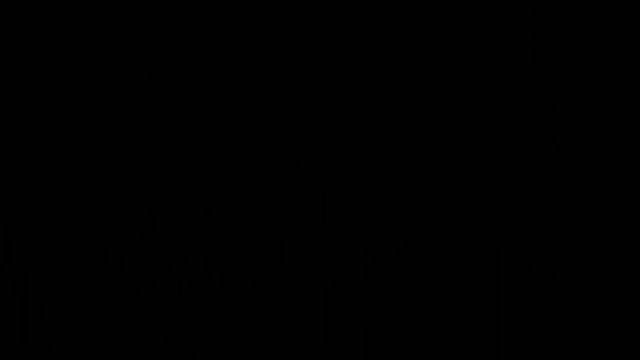 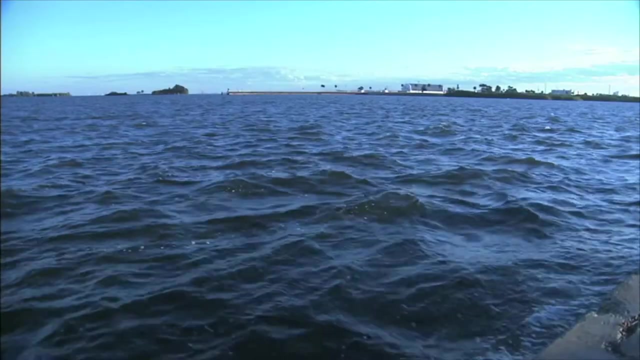 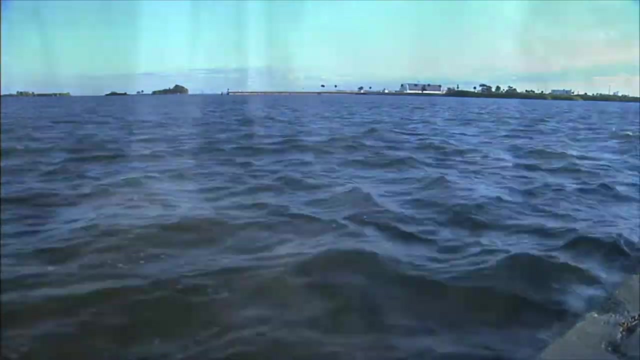 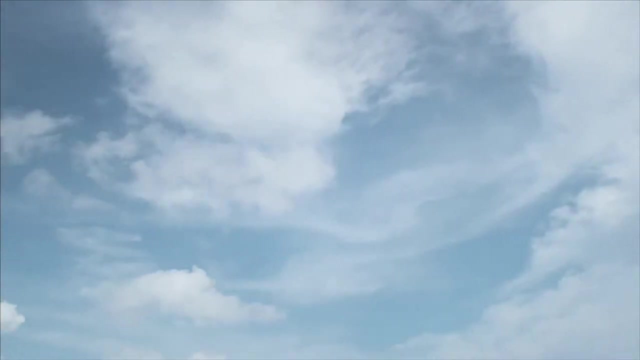 or frost, and sphera meaning globe. The cryosphere is part of the Earth's hydrosphere. The hydrosphere comprises the total amount of water on a planet. The cryosphere impacts everything on Earth: Ninety percent of the solar energy.